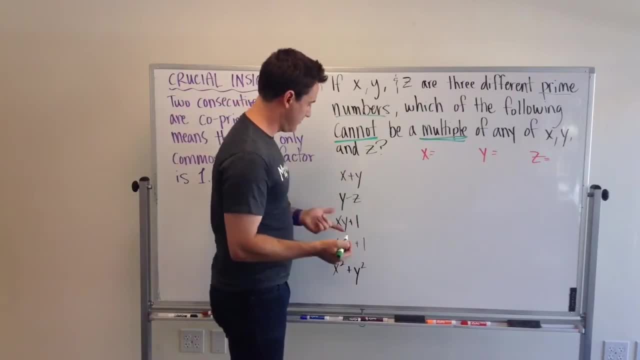 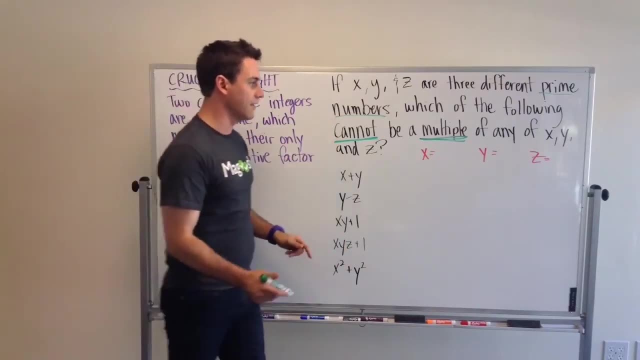 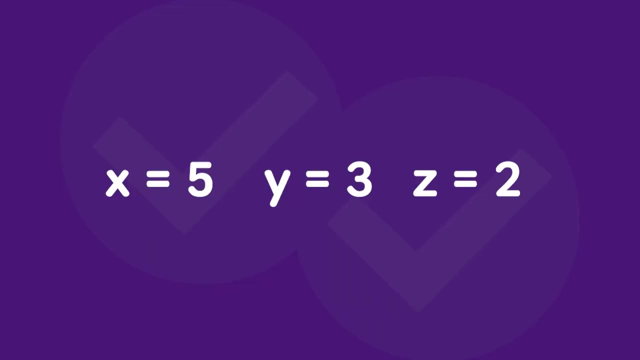 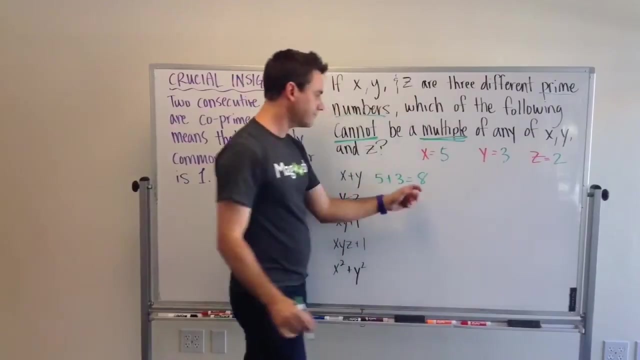 prime numbers for to plug into our answer choices and find which one of these answers is not a multiple of x, y or z. So let's say that this is five, three and two. So x plus y, five plus three, that equals eight. Is eight a multiple of one of these numbers? 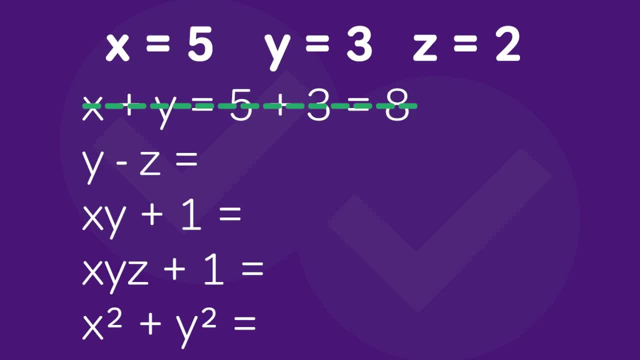 Yes, it's a multiple of two, So we can eliminate it. Y minus z, y, three minus two equals one, And is one a multiple of these numbers? It's a multiple of all these numbers, So. 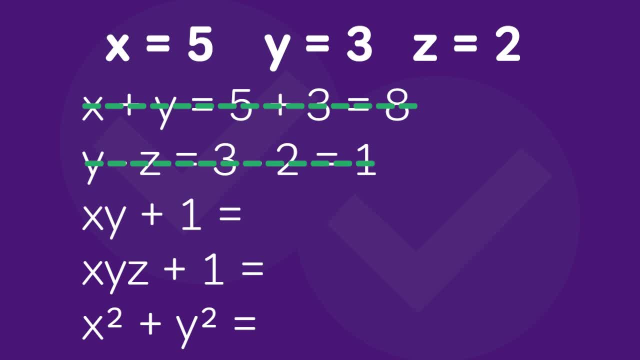 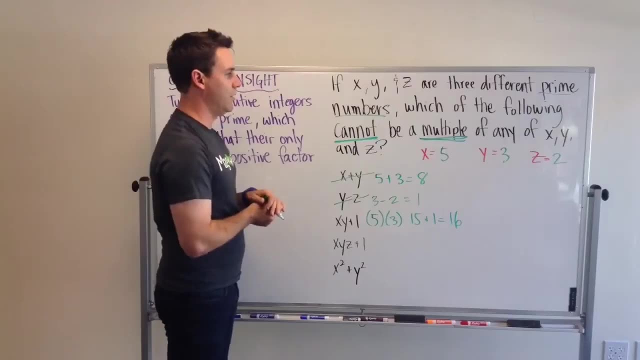 we can eliminate it: X, y plus one, So x times y plus one. So five times three, it's fifteen plus one equals sixteen, Is sixteen. a multiple of one of these numbers, Or, excuse me, is one of: 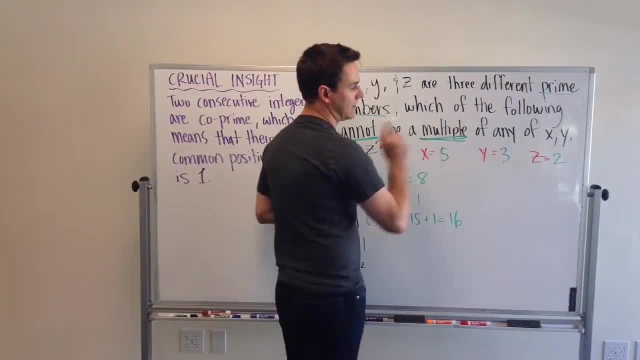 these numbers a multiple of sixteen. I've been saying this wrong. Yes, it's two, So we can eliminate x? y plus one. Now we have x y z plus one, So it'll be x y z plus. 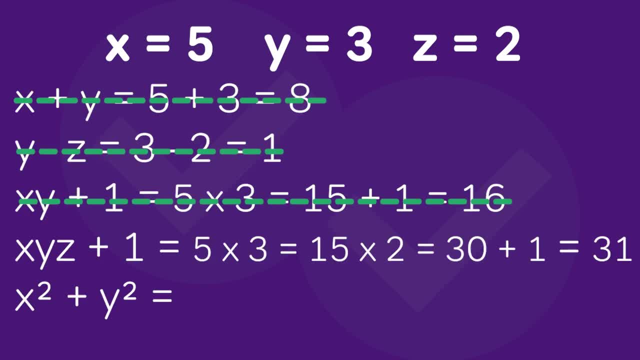 one, So that equals fifteen times zero. Say it, it's. you're achoing a question. Say it all the time. No, it beats you All right. So now we can eliminate y-and-y, So we're. 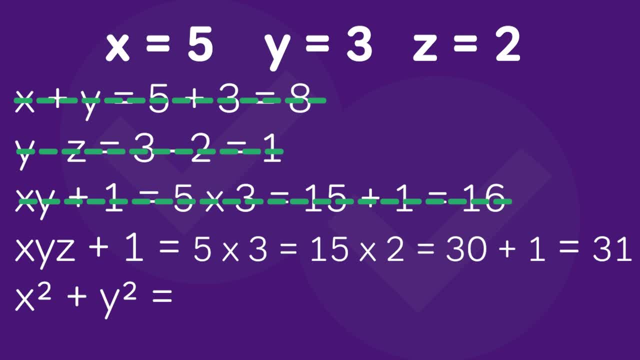 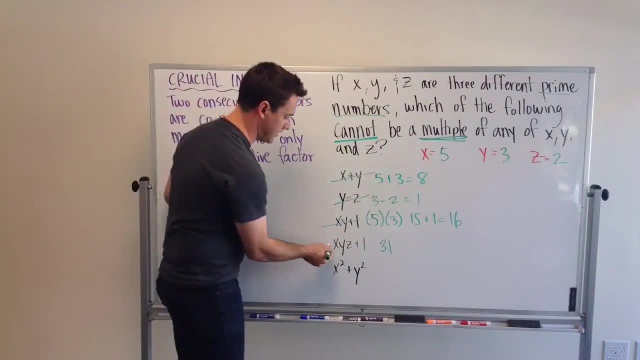 going to could do. if five times three, which is fifteen times two is thirty plus one is thirty-one, Are any of these numbers a multiple of thirty-one? No, All right. so this is looking good. That's supposed to be a star. That's a bad star, All right. One more answer for choice. 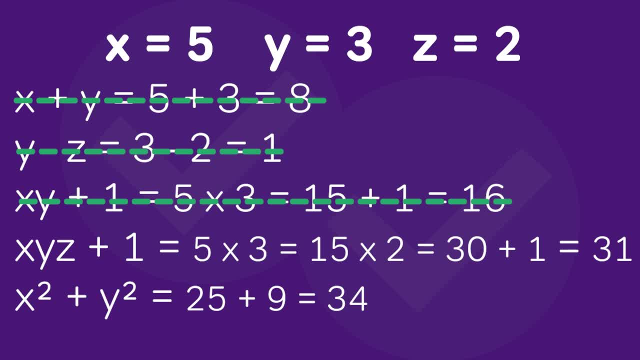 to check: X squared plus y squared, So five squared is twenty-five plus nine and nine. So that's that's beş, All right. Five, six, seven is twenty one. that equals fifteen zero. Are any of these numbers a multiple of thirty-one? No, All right. so this is looking. 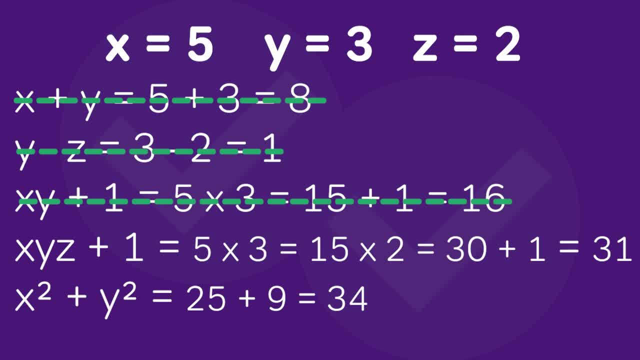 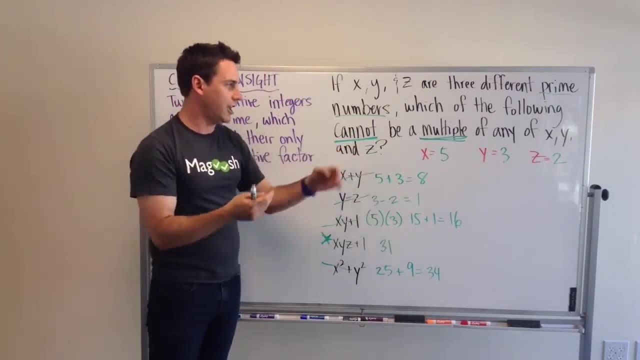 because 3 times 3 is 9 and that gives us 34.. Are any of these numbers a multiple of 34?? Yes, 2 is so we can eliminate it. So this approach can get you to the right answer. I actually 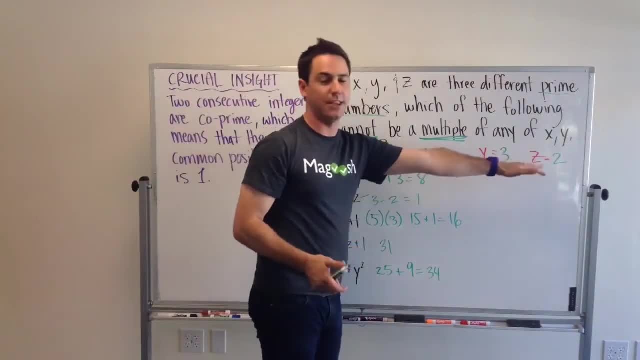 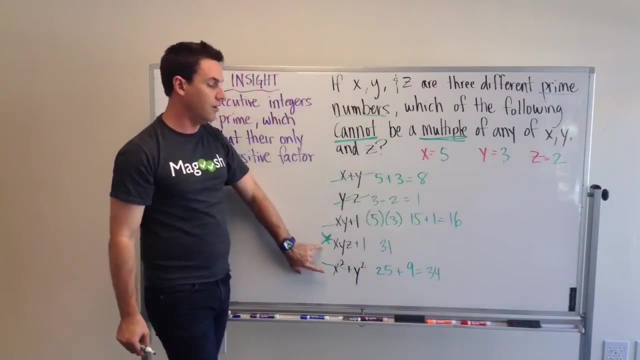 cheated a little bit because I was very smart with the numbers that I chose. If you were to do these opposite- 2, 3, and 5,- you'd end up having these two, which means you'd have to plug in more numbers again to see which of these two is actually not a multiple. So that's going to be. 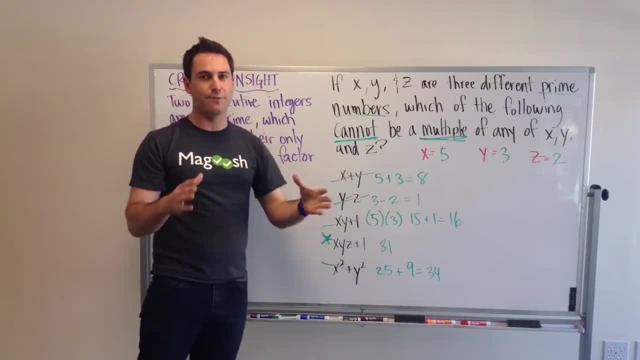 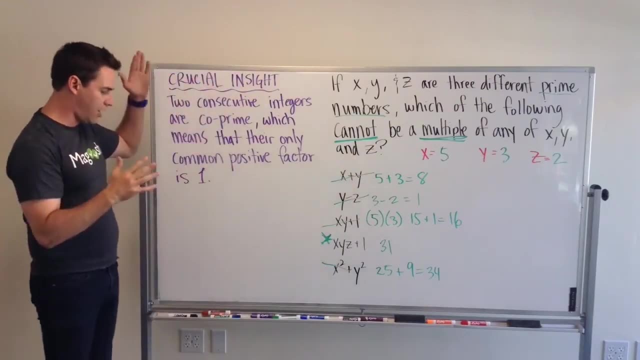 time consuming on the test And the GMAT rewards you for finding shortcuts, for knowing stuff about numbers, And one thing that you should know now, walking away from this video, is what a co-prime is and what that means. So here's the crucial insight. 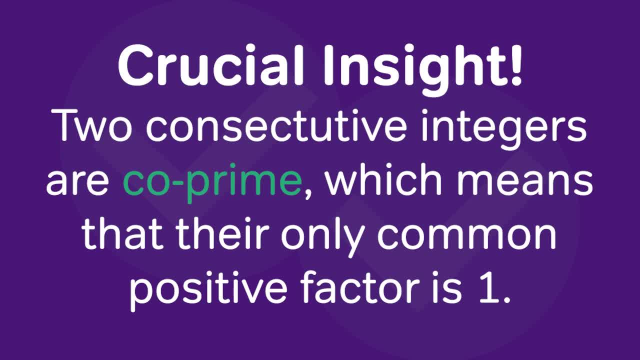 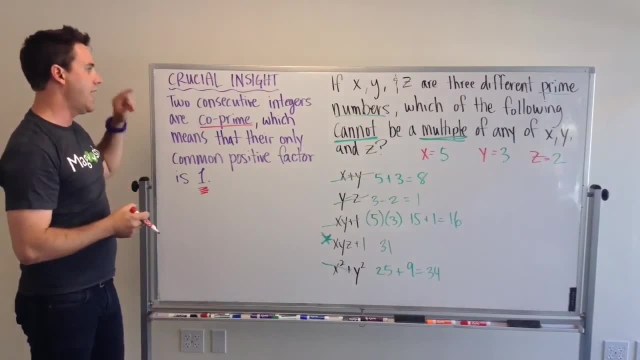 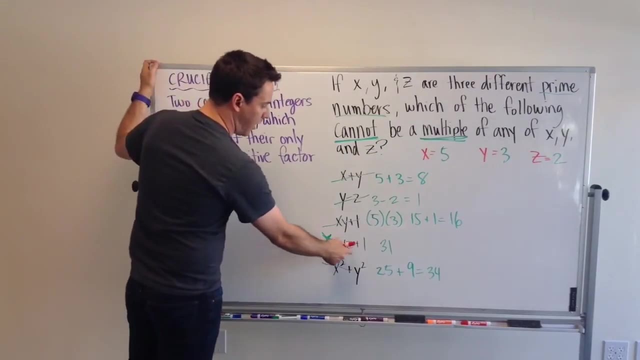 Two consecutive integers are co-prime, which means that their only common positive factor is 1.. Okay, so how does that help us? If you were to look at these answer choices and know about co-primes and know about multiples, you would know that x, y and z. 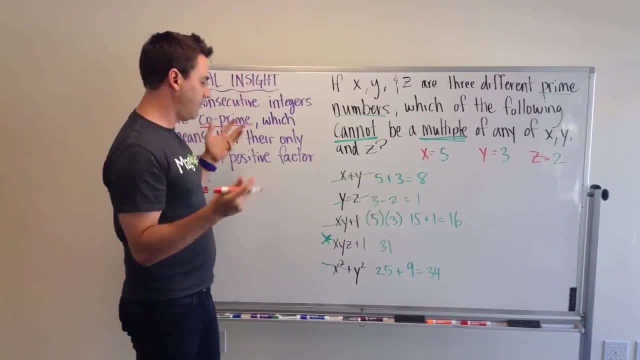 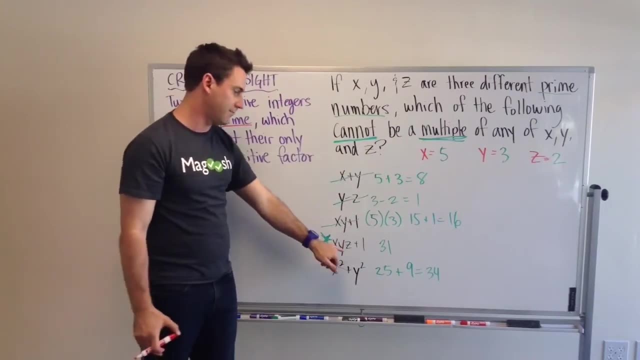 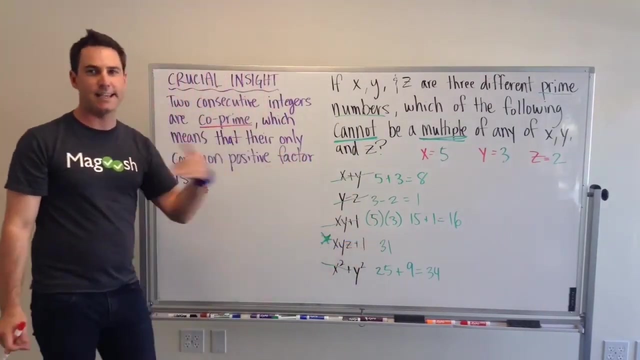 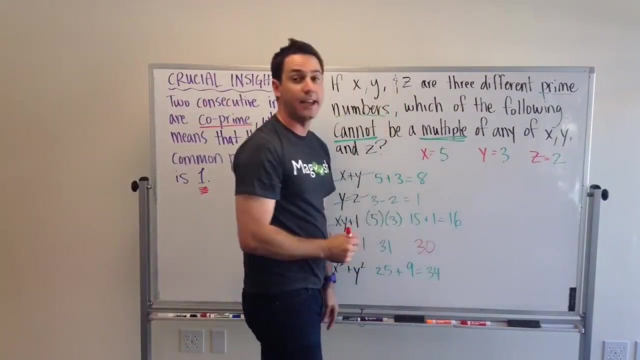 if you were to just have that answer choice, you would definitely have to eliminate it, Because x, y and z is a multiple of x times y times z, But x times y times z plus 1 is the next consecutive number. So in this case x, y and z would have been 30, and then the 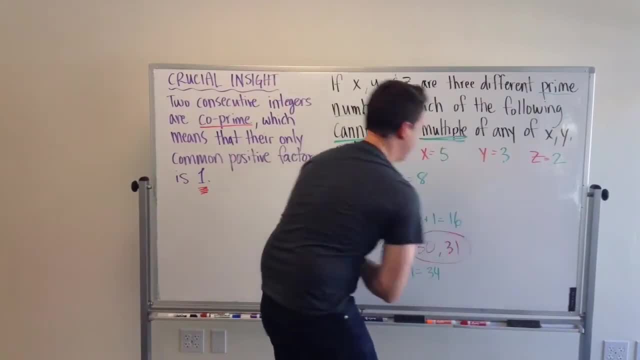 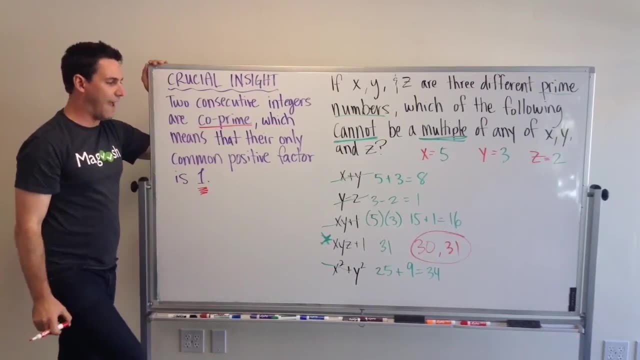 next consecutive number would have been 31.. Looking at these two numbers, you would know, because of co-prime, that 1 is the only common positive factor. So if you were to look at these two numbers, you would know that x is the only common factor. Thus that means that x, y and z. 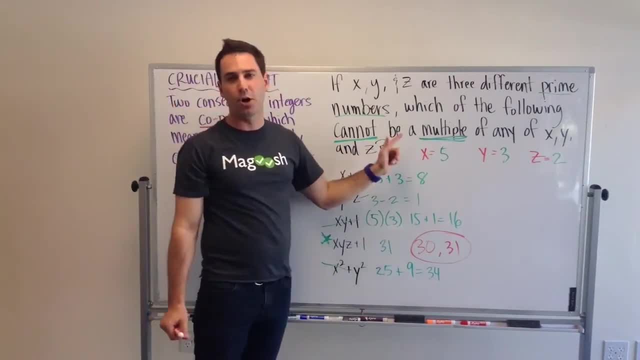 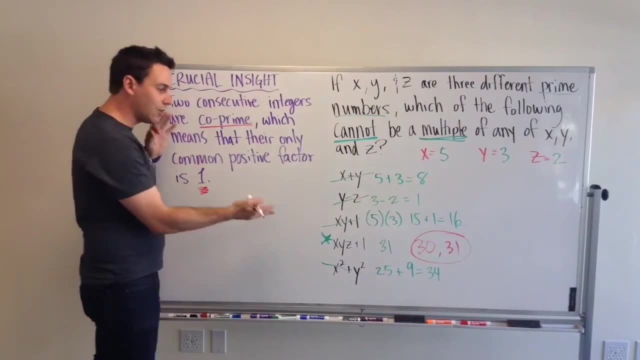 or, excuse me, x, y, z plus 1, 31, cannot be a multiple of x, y or z, So there is the longer way to get to the answer, and then there's always going to be some sort of shortcut. 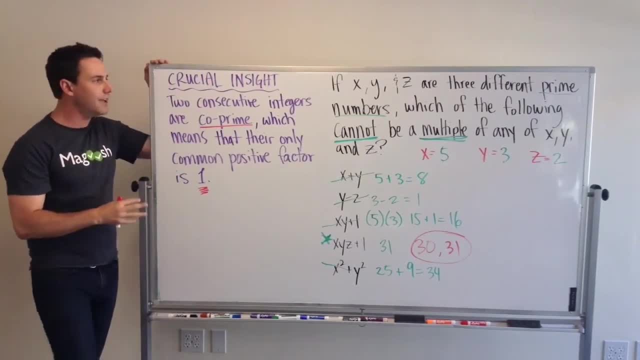 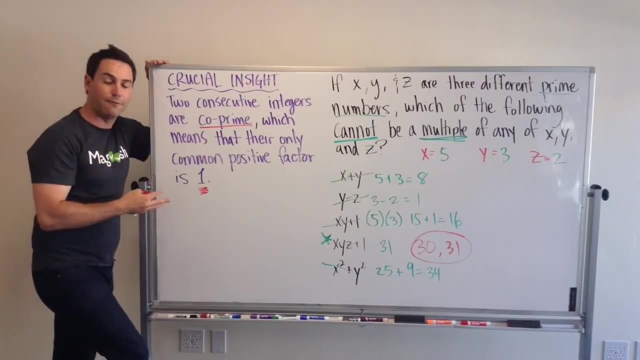 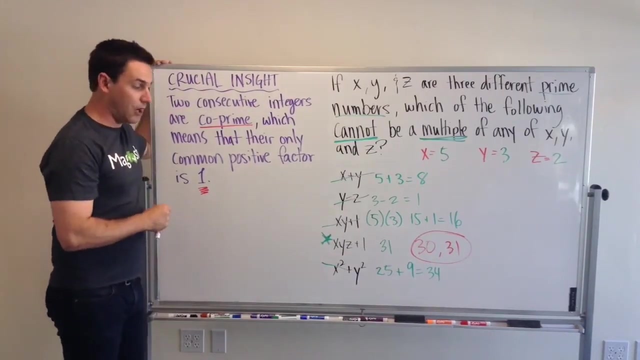 They're going to reward you for doing your due diligence, spending a lot of time understanding your integer properties, understanding the very fundamental basics of integers and number properties. So now, when you approach a problem like this, you can remember. co-prime means.